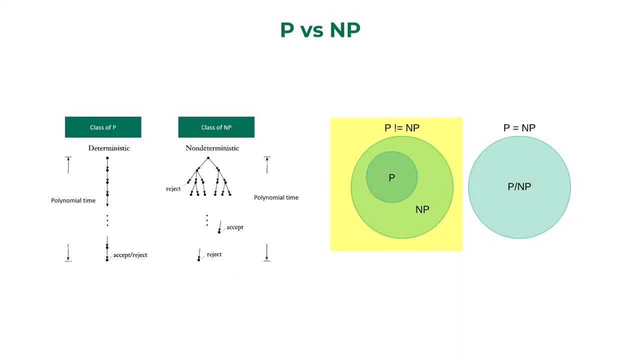 time and P is a proper subset of NP. The other possibility is that P equals NP. There were instances where problems believed to be in the class of NP condensed to P. This is an open problem in theoretical computer science. Now, all the problems that are intrinsically harder than those that can be solved by a. 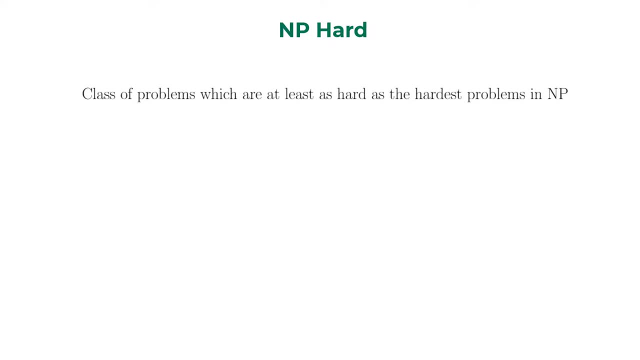 non-deterministic Turing machine in polynomial time are classified to be in the class NP hard. These are the problems that can never be in the class of P, But this sort of classification is too broad as it contains problems that do not even have polynomial time verifiers and also can 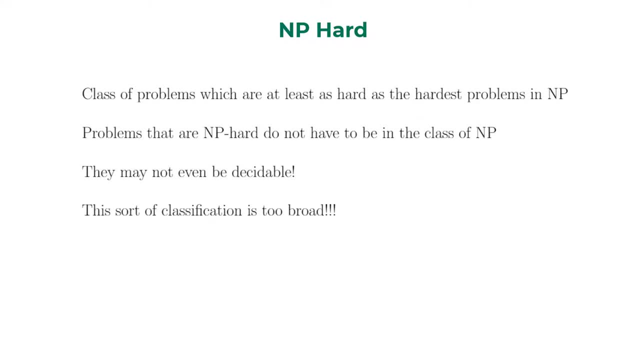 contain problems that are not even in the class of NP. So the problems that can never be in the class of NP are classified to be in the class NP- hard And with the arms in the class of NP. we clearly have the complexity of such a problem. 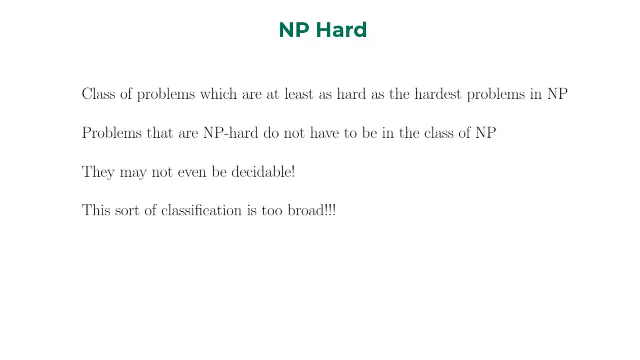 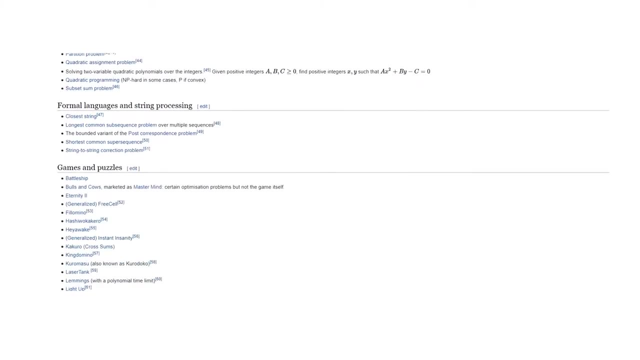 So classifying a problem to be NP hard talks very little about the complexity. Okay, so that one is enough. so I'd like to close this thought for tonight. As many problems of real-world importance are in the class of NP, a better question to ask is: 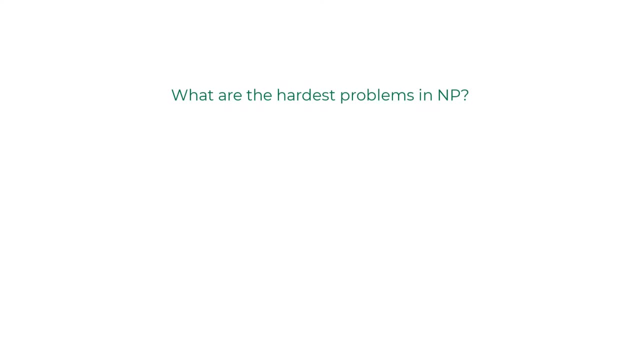 are there problems in NP that are definitely not known to be decided in polynomial time Turns out there are. In early Victorian favorites there were three small basic problems in NP. In the early 1970s Cook and Levin discovered certain problems in NP whose individual complexity is related to that entire class. 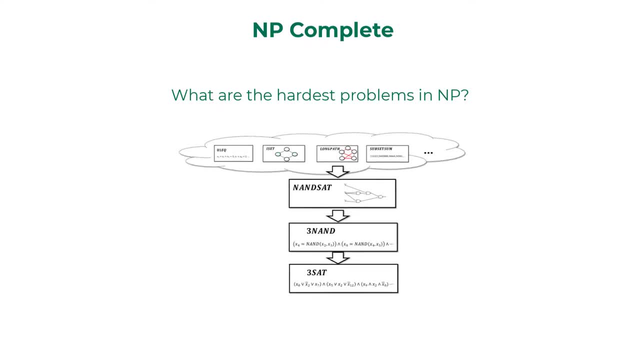 If a polynomial time algorithm exists for any of these problems, all problems in NP would be solvable in polynomial time. Basically, every problem in NP reduces to the special class of problems classified to be in the class of NP-complete. The implications of the class of NP-complete are huge.